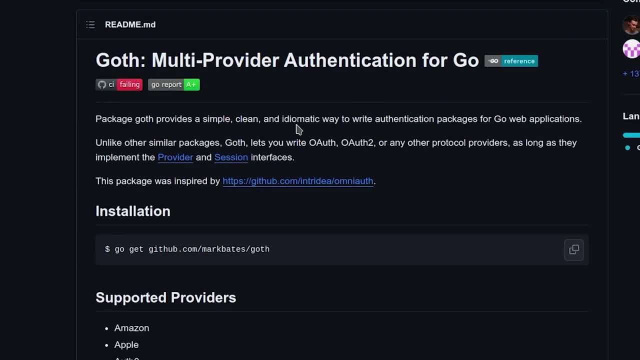 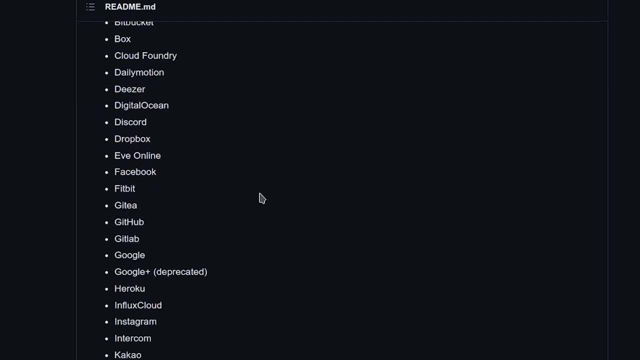 authentication for Go Package. Goth provides a simple, clean and idiomatic way to write authentication packages for Go web applications. You can see here all the support it provides. I mean, they literally have everything: GitHub, EVE online, Okta, Salesforce, Shopify, SoundCloud. 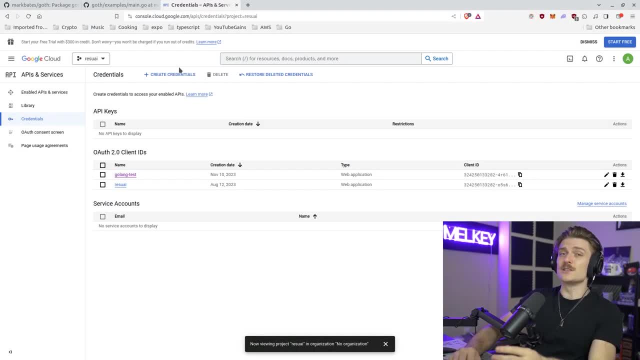 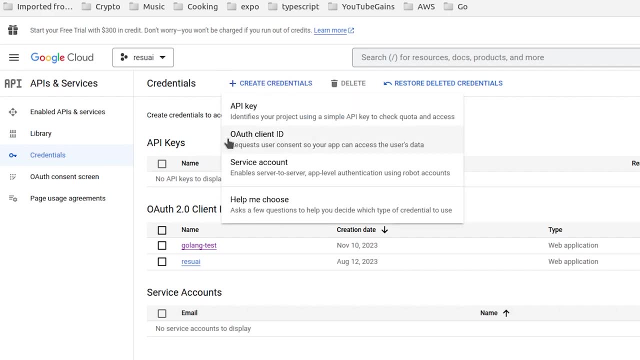 SoundCloud. It has everything, basically. So the very first thing that you're going to want to do is head on over to consolecloudgooglecom, Go to your API library. I'm going to create a new credentials application, an OAuth client ID. As you can see, I have a couple already that I'm 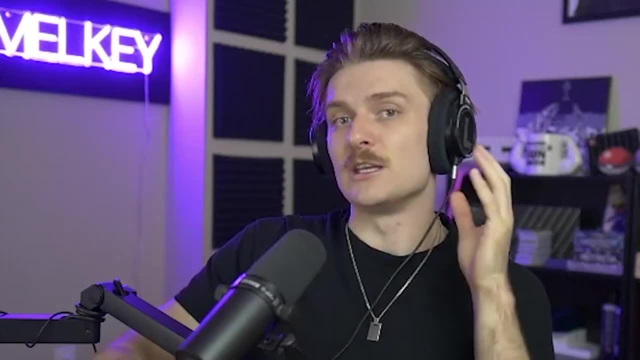 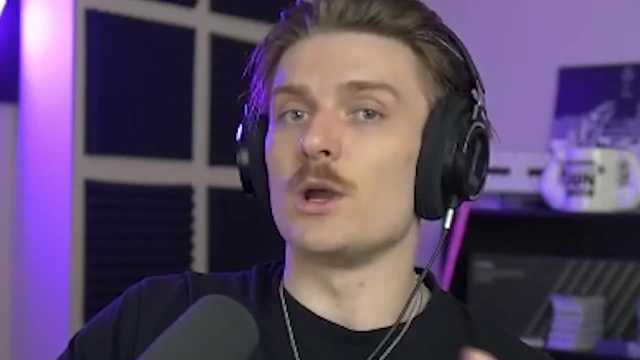 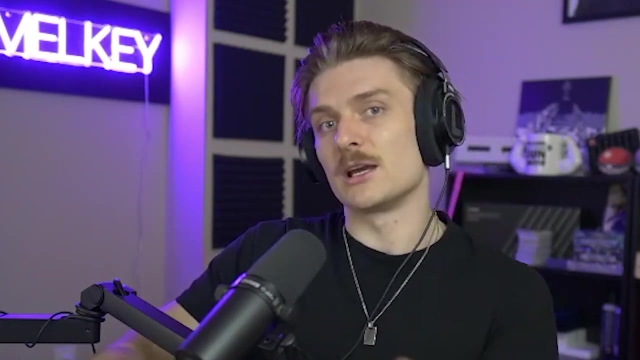 going to use for this demonstration, because this sets you up. It gives you the client ID and secret ID And then you can also set up a callback to localhost 2000 or wherever your server is hosted. Again, this is server side handling, So you want it to be where your server is to hit the endpoint. 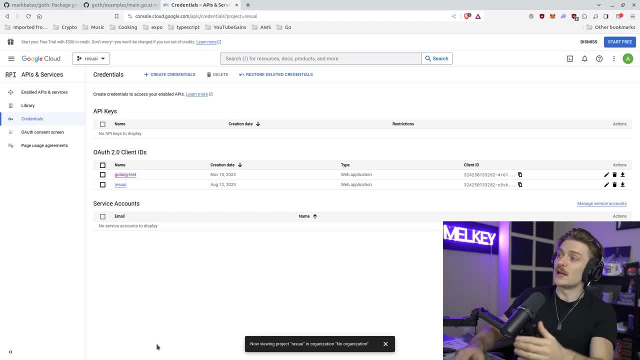 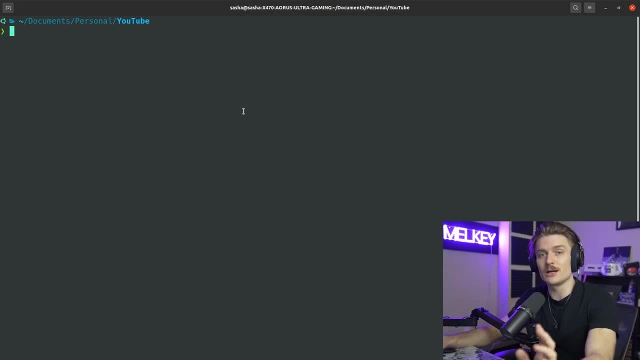 I'm going to show you to set that up on the backend right now, but make sure you get the accurate ANV keys from Google to set this up, because we're going to use Google in this example, All right. So now that you got your keys ready, we're going to go ahead and spin up a new project. 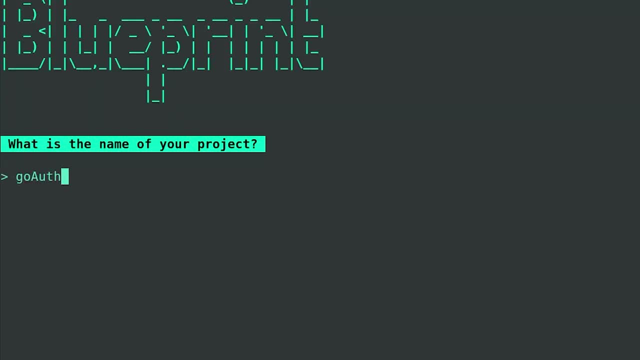 using Go Blueprint Create. The name of the app is going to be called GoBlueprint, And I'm going to call it GoBlueprint, And I'm going to call it GoBlueprint, And I'm going to call it GoBlueprint, And the name of the app is going to be called GoAuth. We are going to use cheat. That's just my. 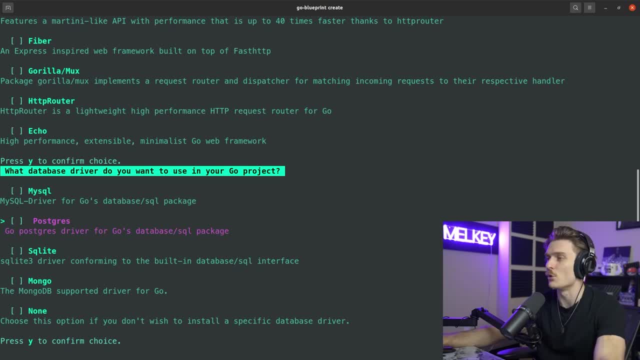 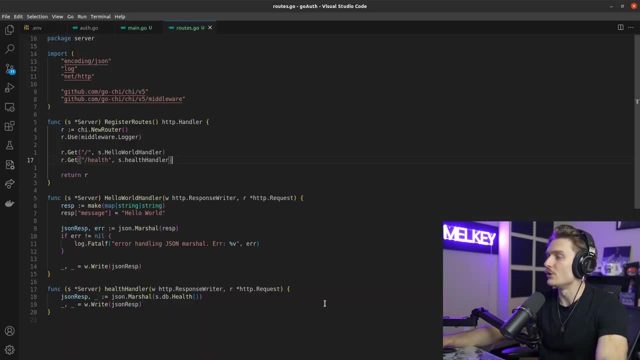 preference. It doesn't really matter what DB you're going to use, but let's go ahead and choose Postgres for this example. Okay, cool, So we're going to cd into GoAuth. I'm going to open up this project And there you go. Now we have a completely spun up Go application ready for us. 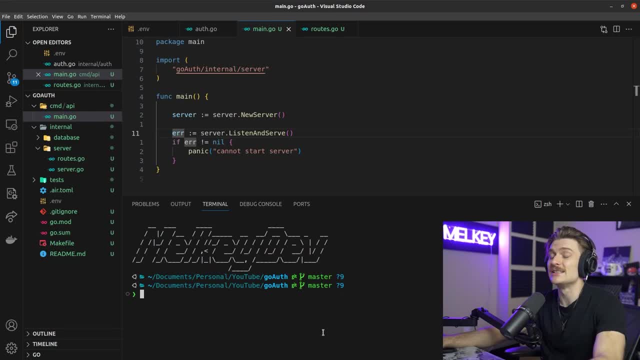 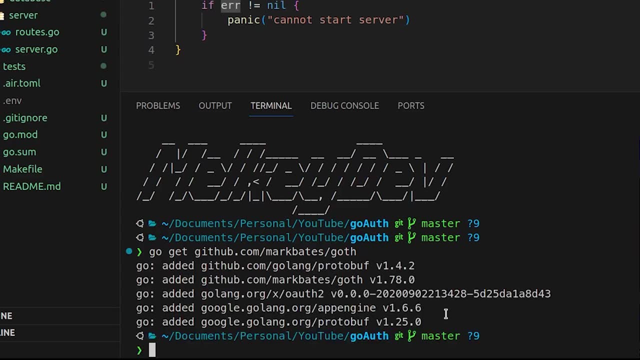 to use. All right, Now we have that set up, We're going to have to actually install our goth package here. You're going to do a go: get githubcom slash, mark Bates slash goth. Just press enter And there you go. 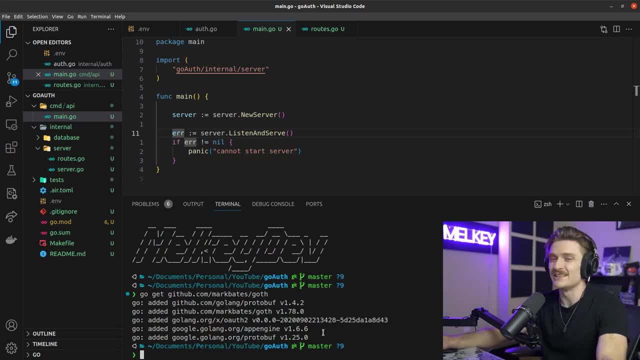 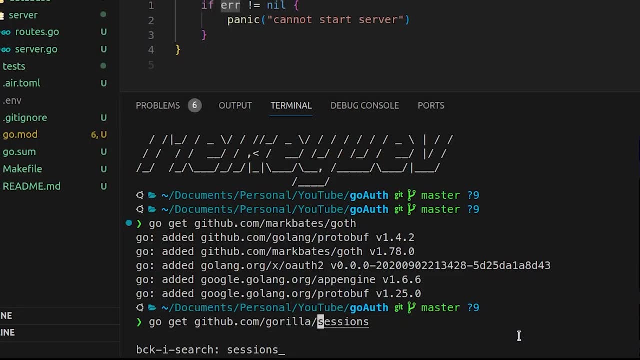 It adds the package for us. It adds an additional Google protobuf, Everything it needs to run successfully. There's the OAuth 2 package as well, And one more is we're going to need the github gorilla session. So go ahead and do go get githubcom slash, gorilla slash sessions. So after 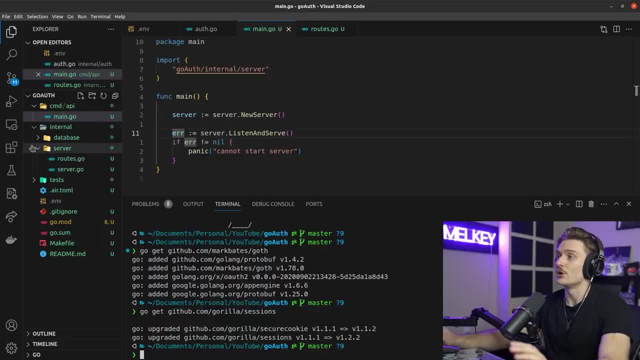 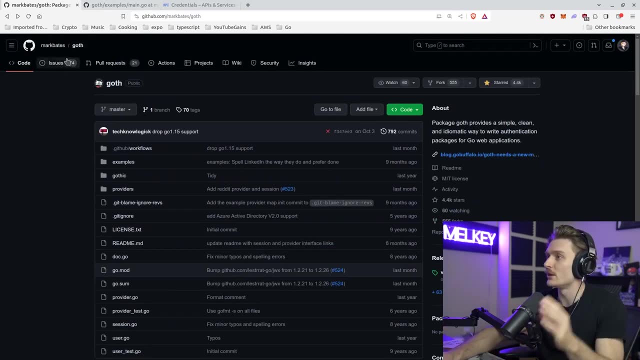 we installed gorilla sessions. we basically have everything we need to start coding and actually getting this to run. But just before we start, I want to share one thing and this should be the go to for everything For goth. it actually has an example folder. It has one file called maingo. 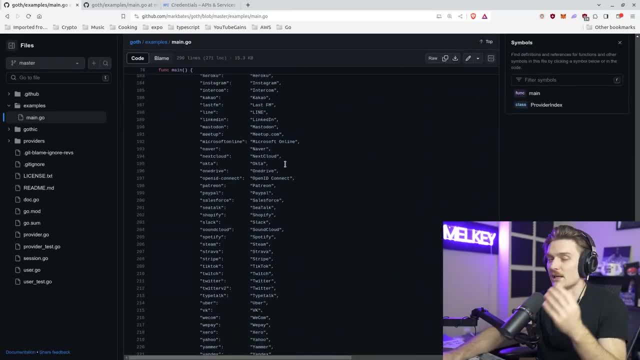 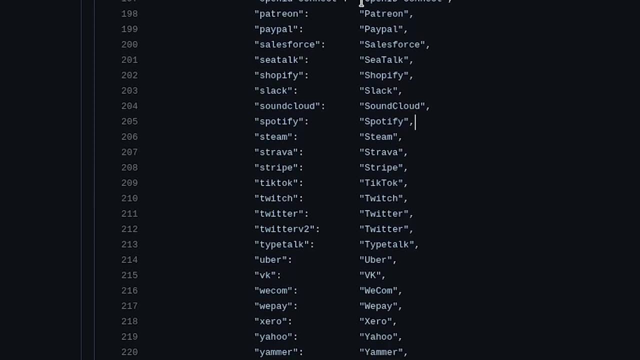 that's going to list everything You need to actually organize and run this with any provider that you want. Like I said earlier, I'm going to do this Google, but you can choose literally any single provider you want And if you ever get lost- this video is not clear- Go to the documentation. go to the example It has it. 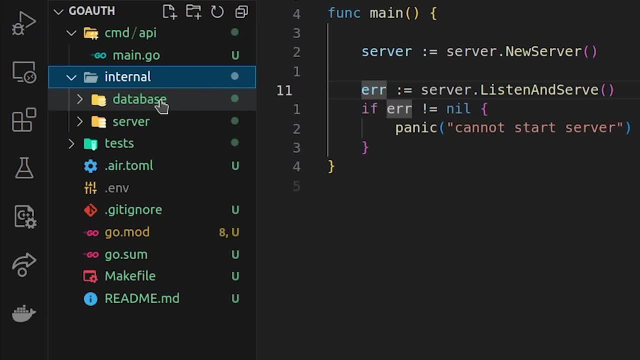 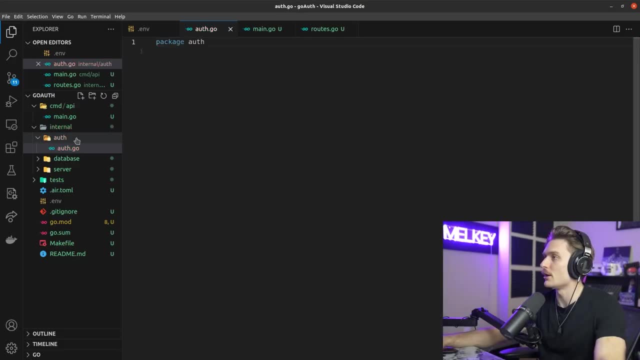 all here for you. All right. So the first thing I am going to do is I'm going to create a new package called auth. I'm going to go and create a new authgo file, Just going to go package auth, And this is basically going to instantiate our gothic store And it's since it's a global- 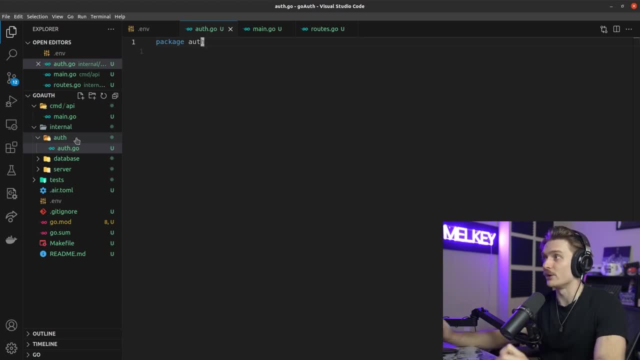 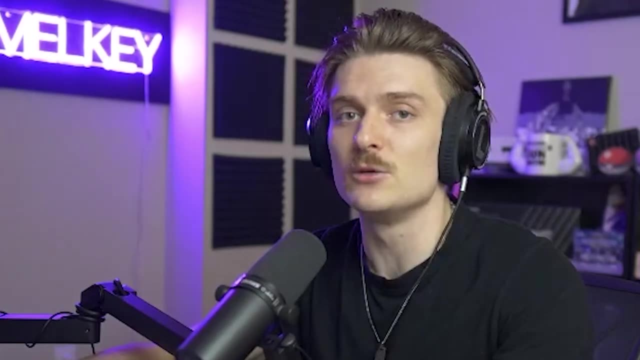 variable a global store. Once we define it in our auth file- here authgo file- and we instantiate it in our maingo file over in cmd slash API, right here, we can basically use it throughout our application code. All right, So let's go ahead and start with our package: auth file- here The 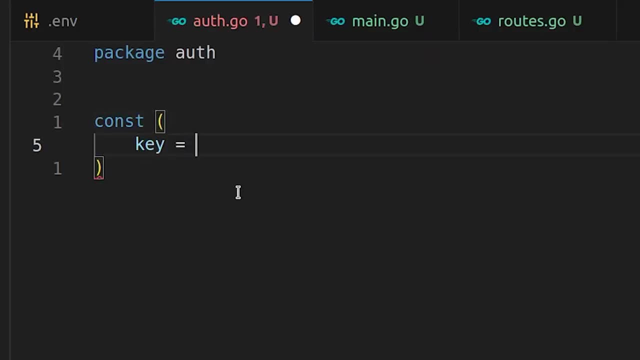 first thing we're going to do is create a few constants. here We're going to do a key, So this is a signing key. You can do a random string. make it definitely more secure than random string. Our max age is going to be 8640 times 30. I think this is 30 days, if I'm not mistaken. 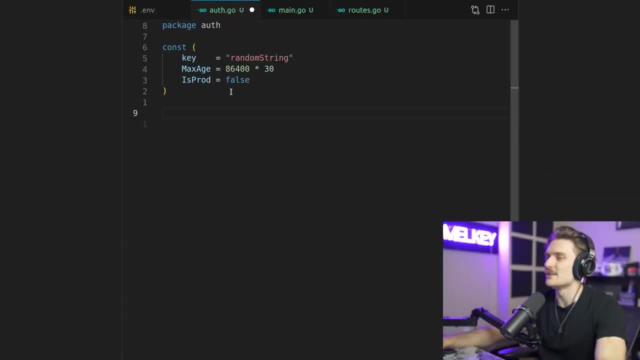 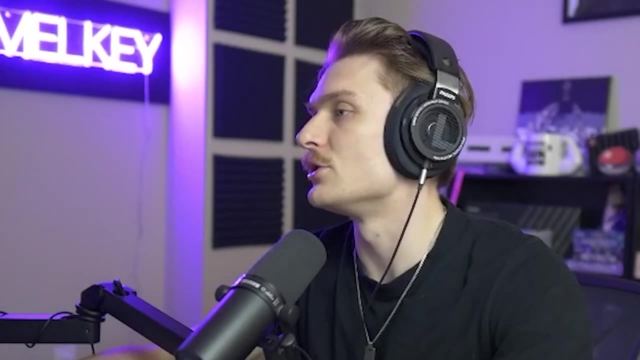 Then we're going to do an is prod variable which basically declares our- is this a production or is this still in development? And then we're going to create a new function called funk, new auth, And this is going to be the constructor, or what's going to get instantiated for our gothic store. 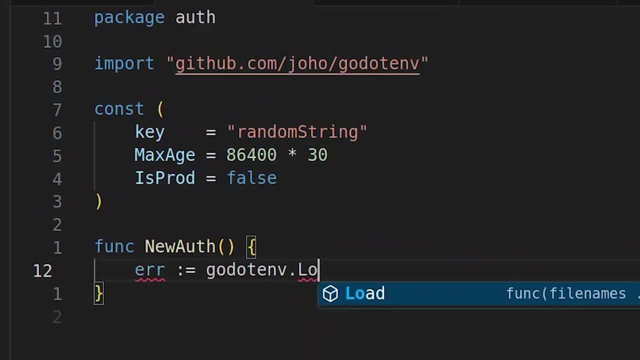 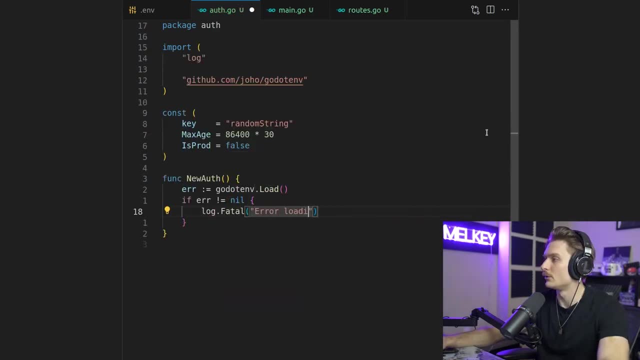 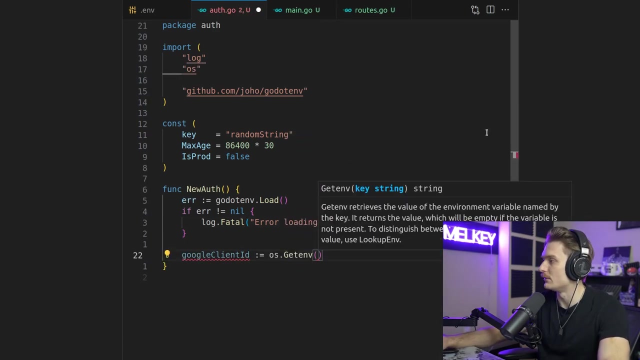 First thing we're going to load up our goenv, our environment variable, So go load. if error does not equal nil, We're going to do log: fatal error- loadingenv file. Next, I'm going to declare my Google client ID, osgetenv. Google client ID and copy this and just put Google secret and then Google client secret. 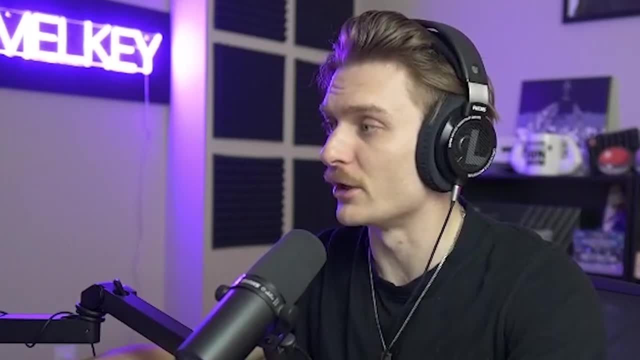 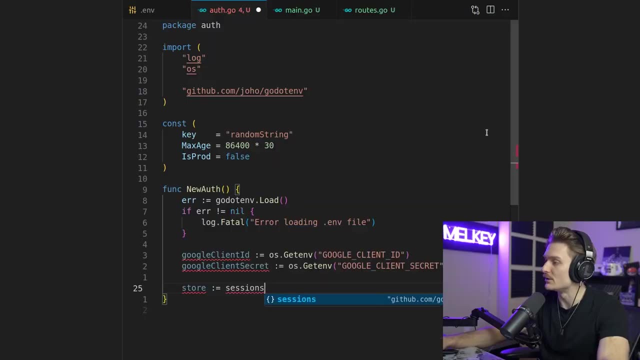 All right, cool. So all we've done so far is load our secrets from our env file using goenv. Next up, we're actually going to declare this store exactly how it's written in the documentation. We're going to do sessions from gorilla sessions. I'm going to do new cookie store. It's going to take. 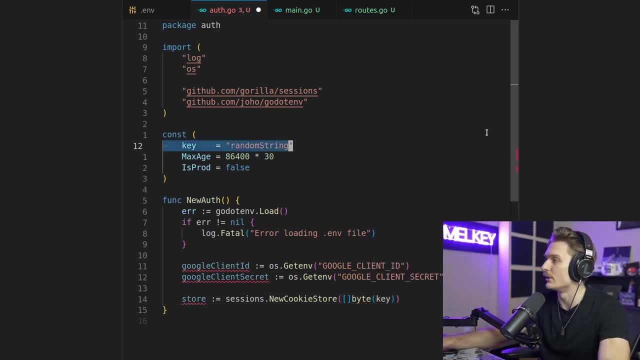 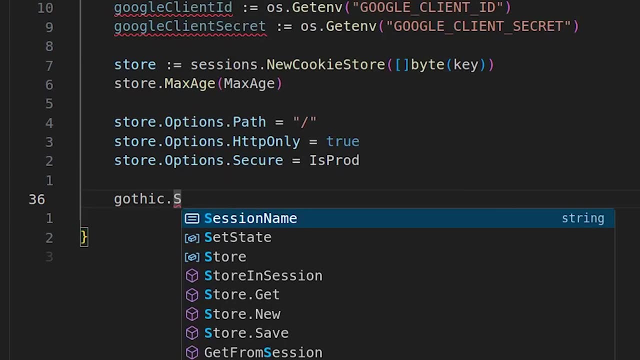 byte of key, our hashing key, which is back online, 14 over here, Now that we have our store, which is just from gorilla sessions, all we're going to do now is bring in our gothic package here, So gothic store, And then here we're actually going to. 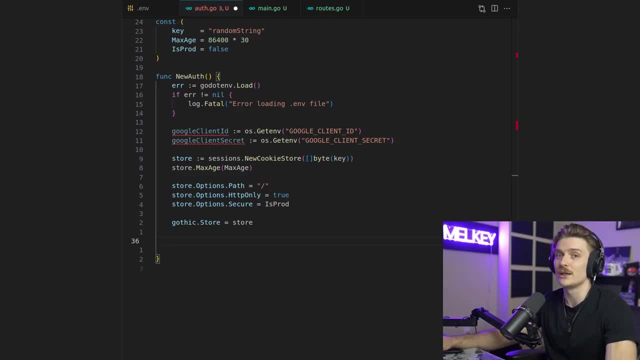 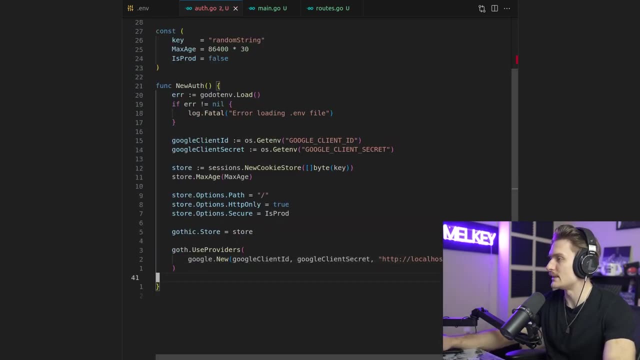 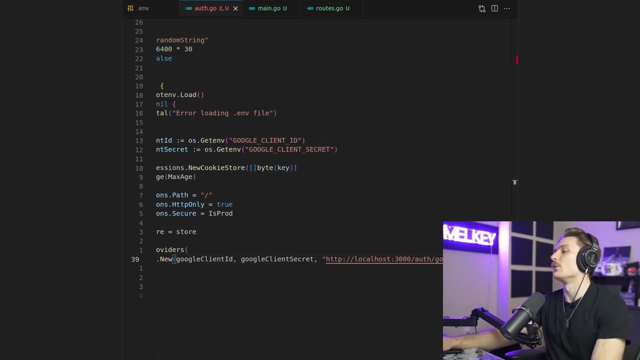 provide the list of providers that we want our application to accept OAuth connections. In this example, we're going to use Google, So we're going to do gothuse providers. We're going to paste in our Googlenew with our Google client ID, our Google client secret and the callback for our 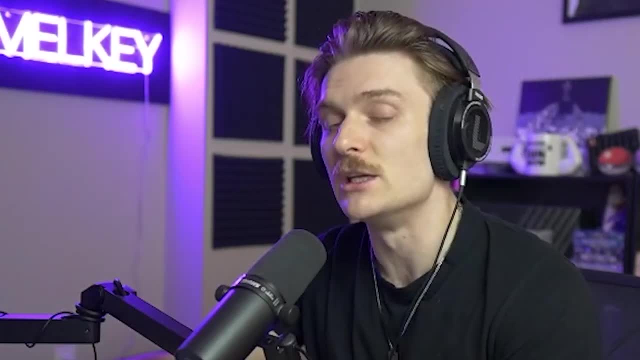 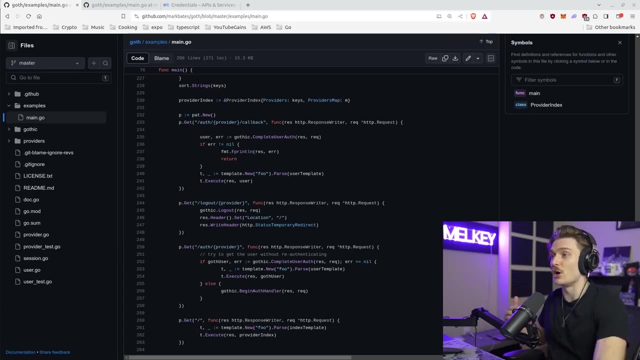 reader, And this has to be the exact same thing You created in your Google client API page, which I showed at the beginning of this video. All right, So now that we have our providers running in gothic and we're going to instantiate. 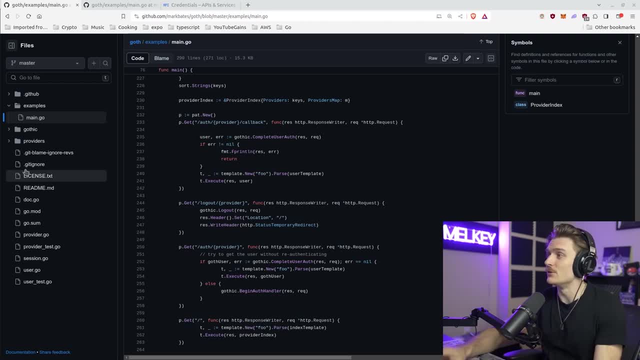 it with our new auth in our maingo file. The next thing that we need to do is actually grab these three routes from the example, from maingo, from the goth repository. What these three are responsible for is actually the callback that triggers the handshake between goth and the 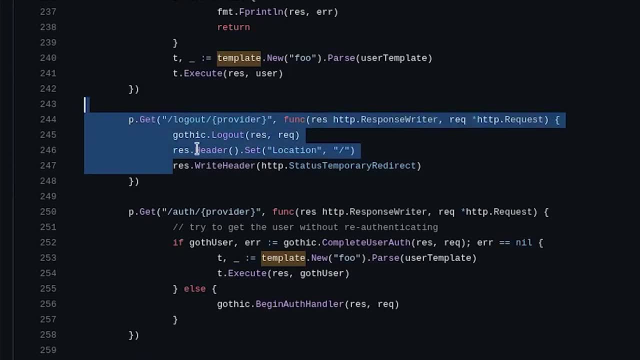 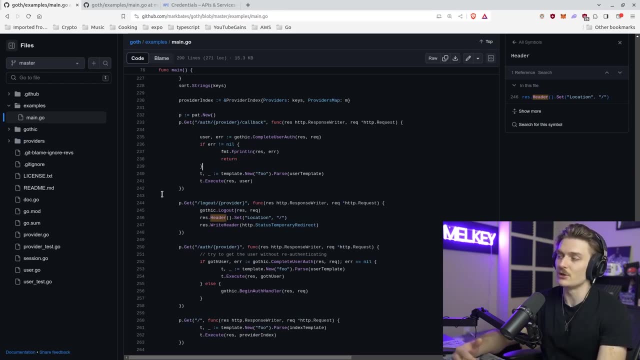 OAuth provider or whatever provider you choose to use, And then, obviously, this is the logout path here. So, because I'm using chi as a middleware, when I ran my project at the beginning with go blueprint, there's going to be something that you're going to need to include If you want to. 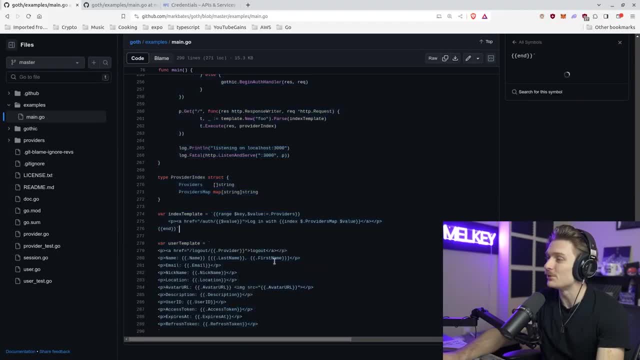 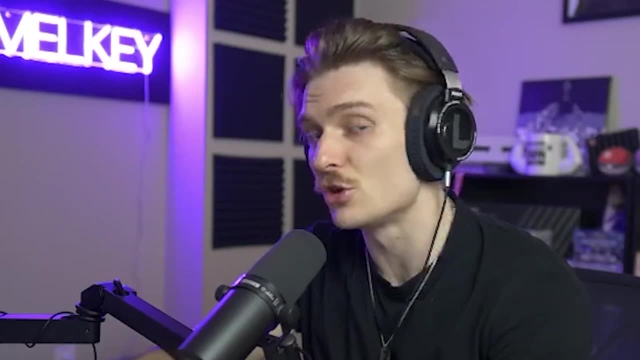 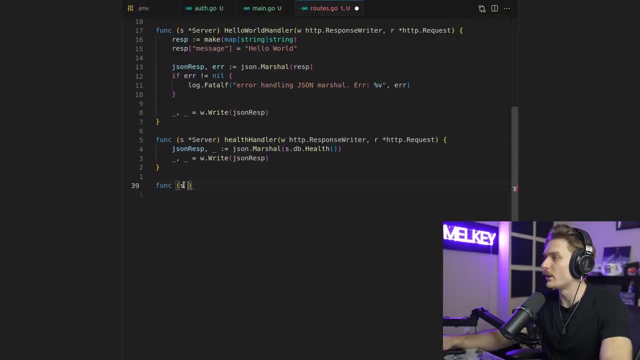 use chi in your project. the example they have here simply uses templating, So they just write HTML and they generate from their server. I want to use chi as just my backend router in go, And then I'm going to spin up a V React app on the front end. All right, So let's go ahead and write. 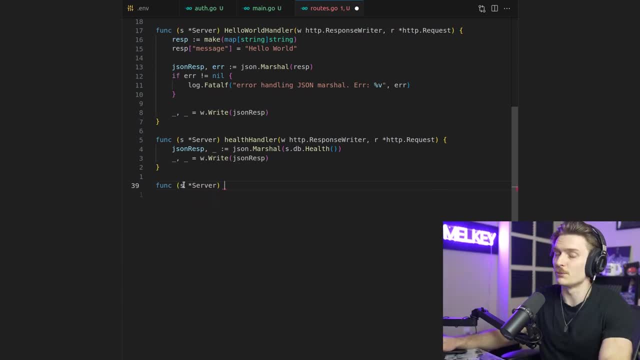 this one out. So I'm going to write out the main callback function and put the other ones- I'm just going to paste them just to save time here. We're going to call our first function getAuthHallback function. It doesn't really matter what you name it, It's going to take our classic HTTP response. 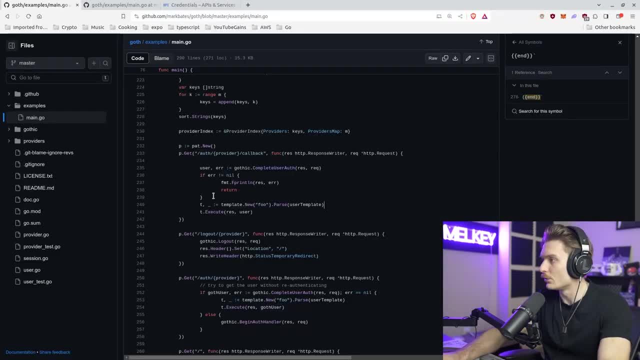 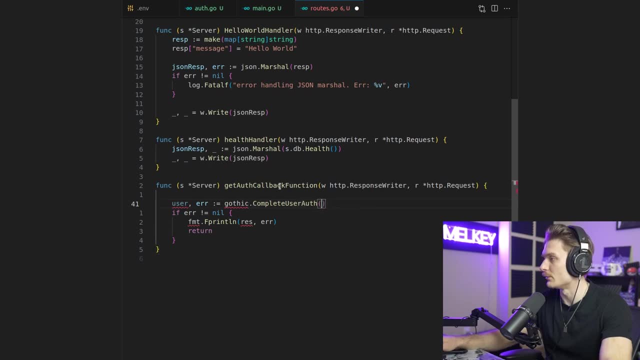 writer and our HTTP request. And then we're going to just basically copy this block of code here from the examples, We're going to paste it here and change this up here, because we don't have res and request, We have w and r, And then all we're going to do is fmtprintln user And this: 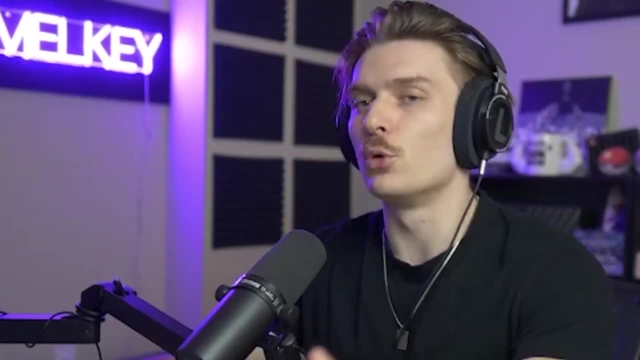 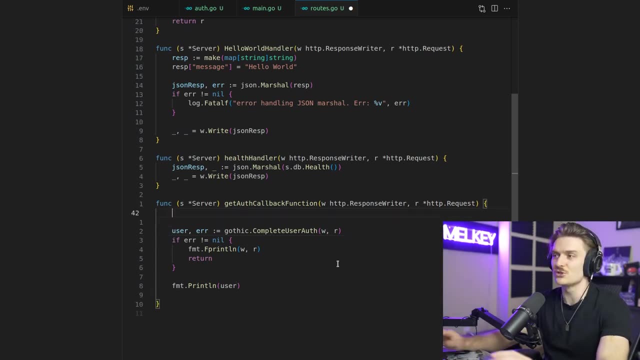 will give us our user information, But I want to give you guys a little bit more than just that. I said earlier, this is actually not going to work. if you use chi, If you spun up your project, you can go blooper, And it's not just chi, It's not going to work. with gin It's not going to work. 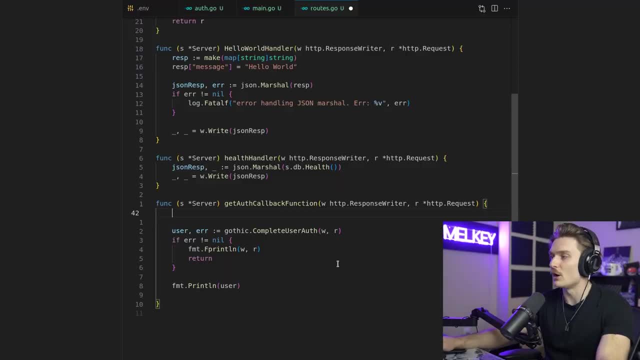 with any of these middleware packages, because the way the context is passed and the way goth looks, you actually have to do a little bit of tuning. So the first thing you want to do is create a variable called provider. You want to do chiurlparam r and then provider. So basically, 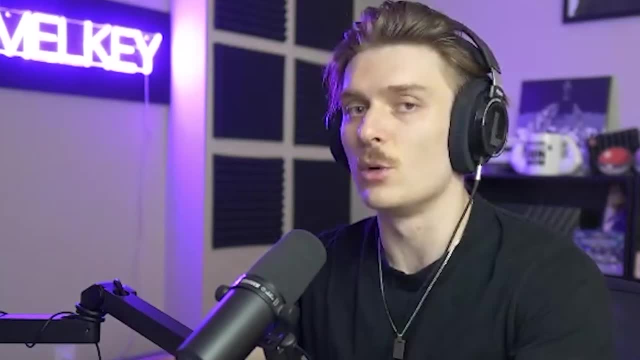 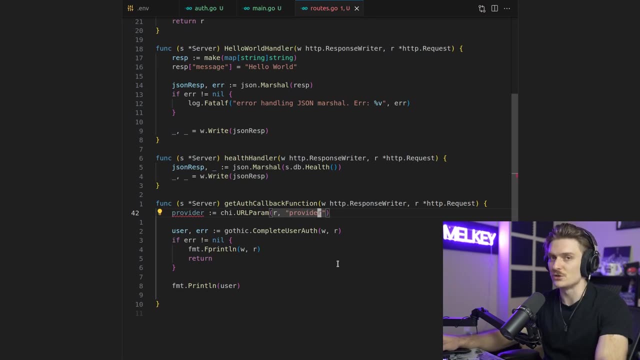 what this is going to look for. the URL parameter provider. If this could be anything, you want to be Google, it could be whatever. I'll show you how we define it in the routes above, But basically this can be a placeholder for whatever the provider you choose to use. 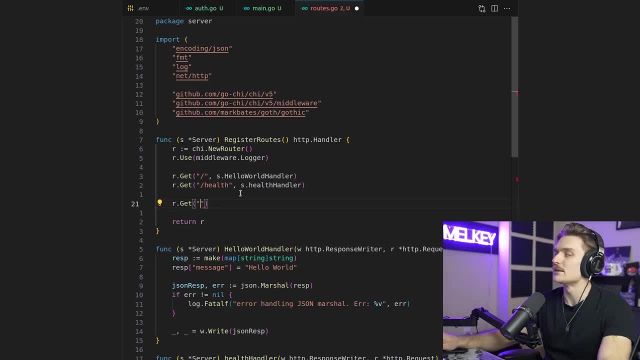 So I'll show you what I mean. if you do an r get right, And then you pass in the route for this provider callback is going to live, It's going to be slash auth, slash provider, slash callback, And then the function is going to be the get callback auth function. So basically now this factor here. 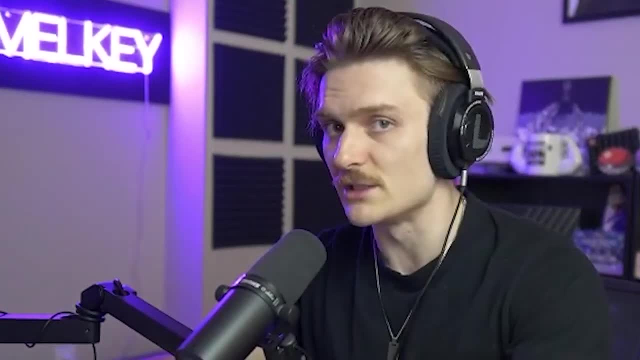 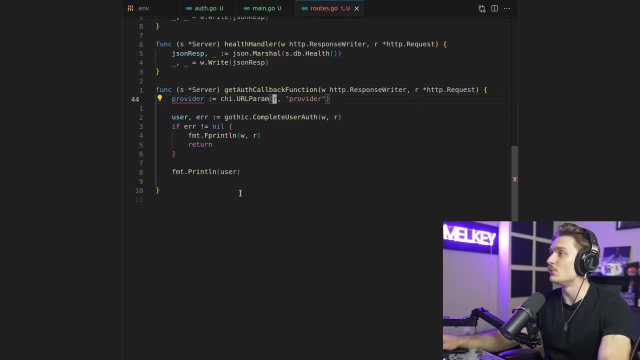 this value here. this you don't have to change, Whether you change from Google or Discord or whatever provider, you can leave this the way it is. However, we need to create this provider variable to pull in that provider link from our actual URL parameter, And now this is not done. 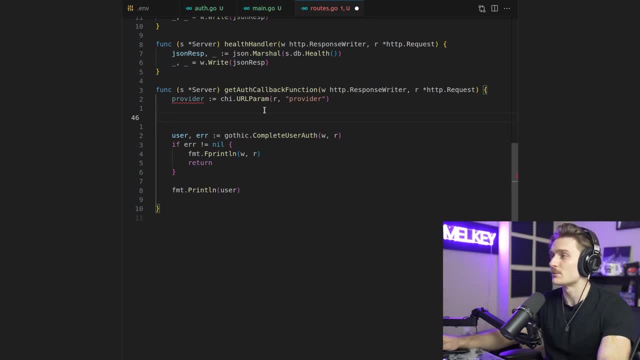 We actually need to modify our, our ruler, our HTTP request pointer, because this needs to be passed into what this provider variable is, And we can do that with our dot, with context context, with value context background, or, if you use an existing background, you can use that. That's fine. And then here we can pass in provider and the last one will be provider. Okay, Awesome. So if you use this, this will work. but there's one more thing I want to include. Whenever you do get auth callback function, you want to redirect your user. You don't want them to just stay at that page, because 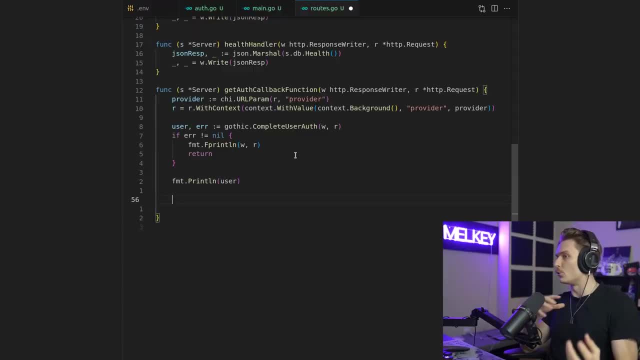 nothing is going to happen. You always want to redirect them back to the route or whatever page you want the user to go to after they successfully log in, And you can do that easily with the HTTP redirect method to W? R and this path, local host, and then the path that you 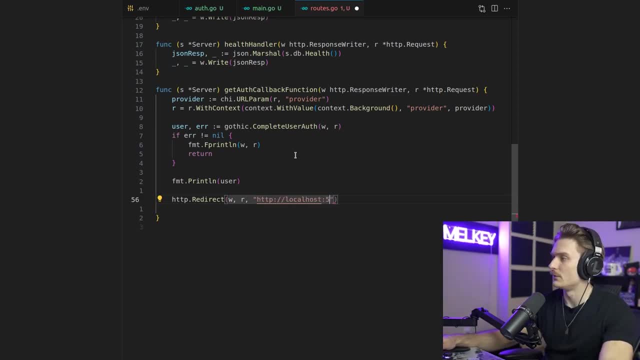 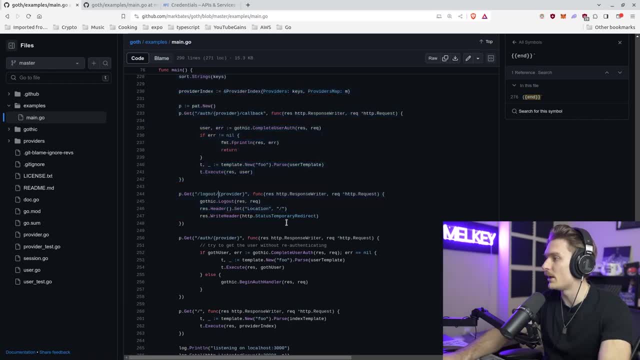 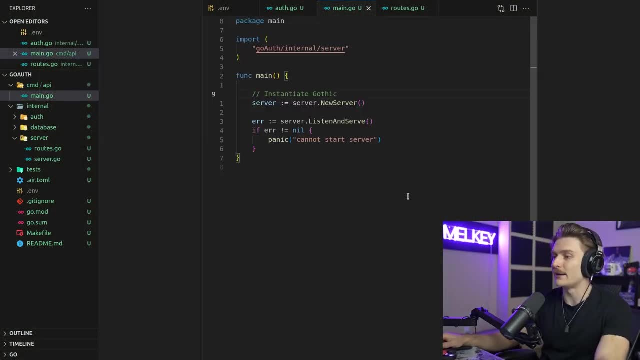 go back to our example here, And we're just going to basically copy and paste the logout function and the auth provider function as well. Now we are almost dumped. Let's go back to our maingo, where we have to instantiate Gothic. So up here I want you to go, bring in the packet. 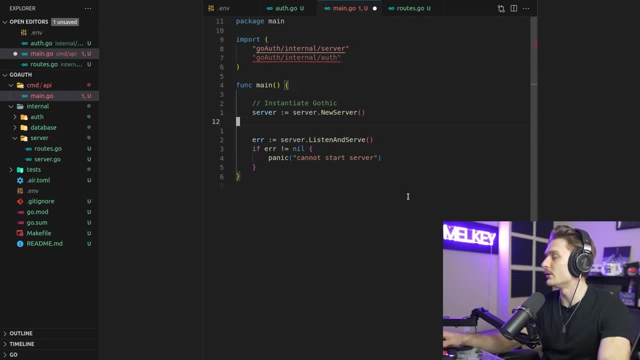 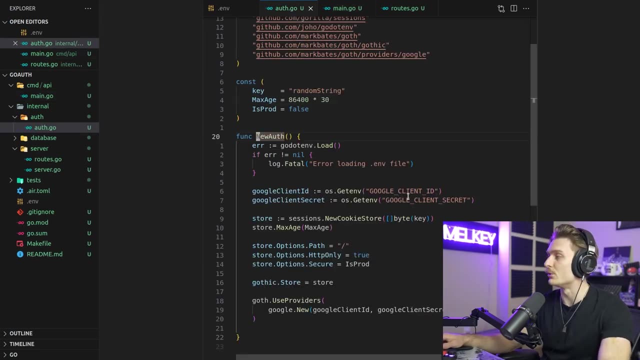 our internal package we created earlier, So internal auth, And then here what we're going to do is auth dot, new auth And that's it. If you follow this, remember this just pulls in our environment variable, creates our store from the sessions. 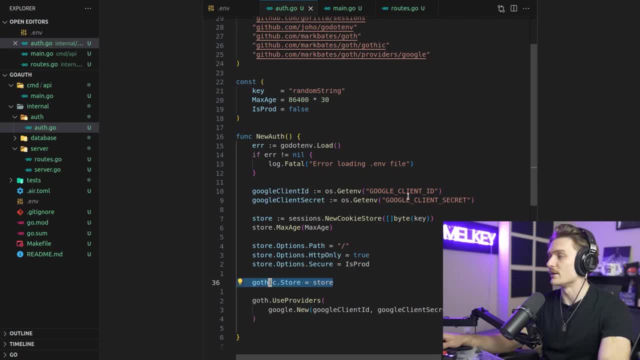 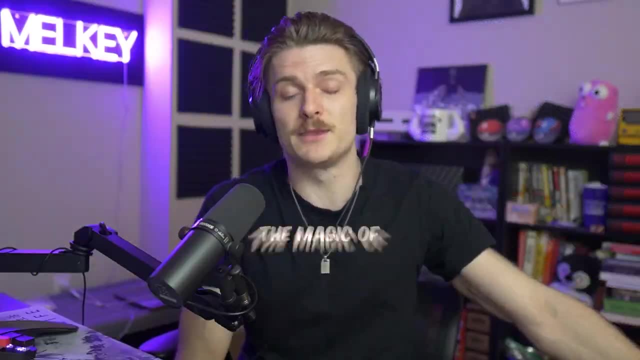 gorilla sessions new cookie store and then puts it into our Gothic store, like so, and give it our list of providers, which our application will accept. All right, So we have gone through what the magic of go, auth or goth is going to be. I've 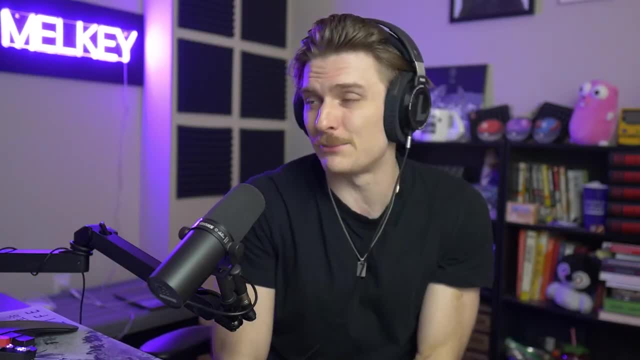 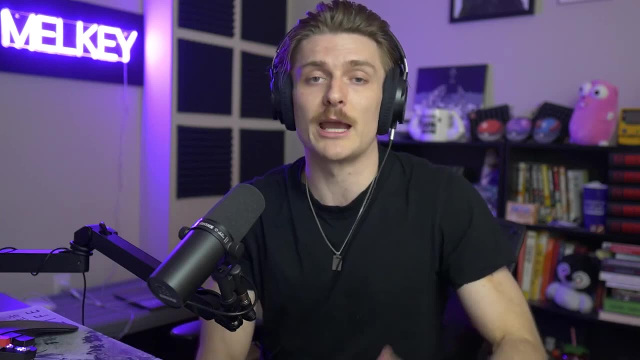 explained a little bit of authentication. I've even showed you how to basically spin up an application with auth here. but now I want to show you how you can actually use this with a front end. We're going to quickly spin up a TypeScript react project. We're going to 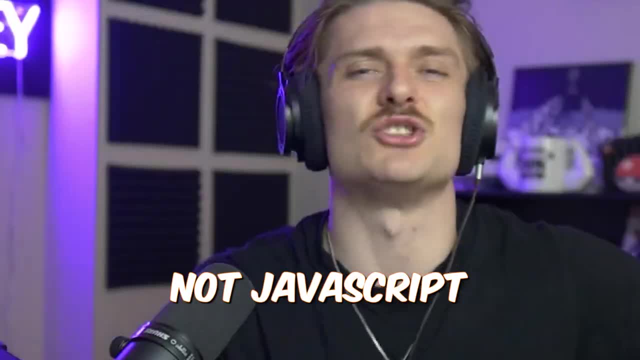 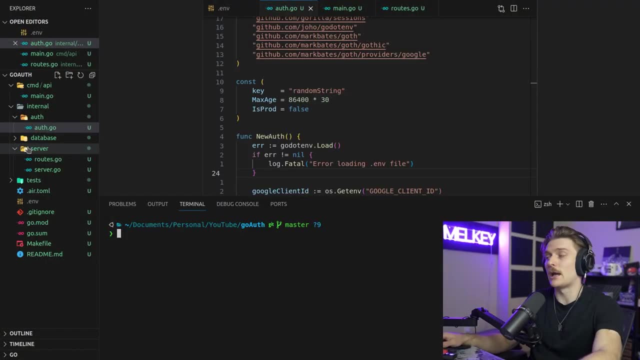 modify it just a teeny, weeny bit, because we're Golang developers, not JavaScript, TypeScript developers. but I'm going to show you this end to end flow. So stick around right now till the end. Okay, So I'm back in my application. You can see here I didn't do anything behind the scenes, It's. 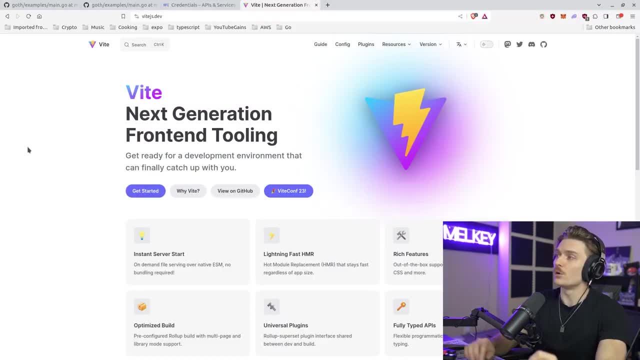 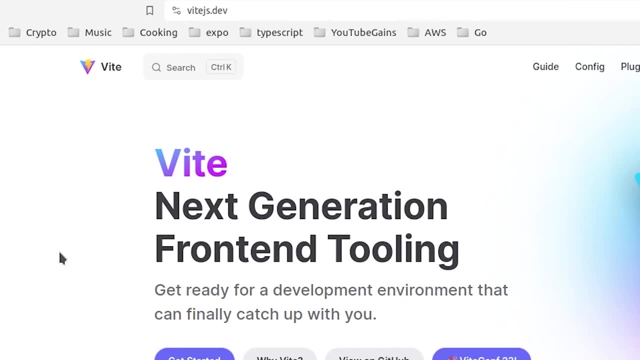 the exact same. Everything runs as expected. but now we're going to use Vite, which, if you haven't heard of it, is this tool that spins up front end projects using react. You can choose what language if you want to use react server components. it's really, really neat. It's pretty lightweight. 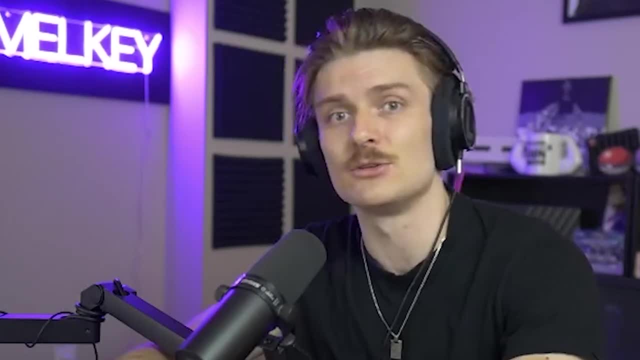 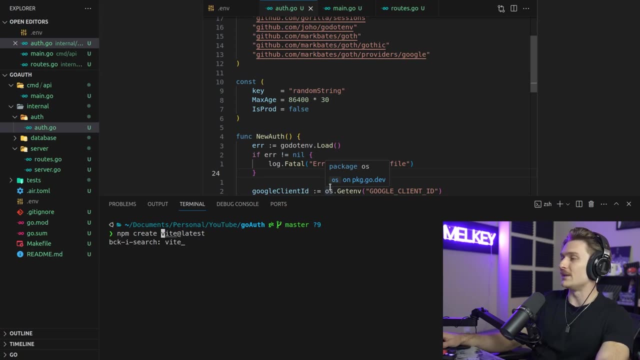 You know, if you don't need something like next, you just want a front end to do front end things and you hook it up to a back end. I think this is really the most vital option to you. So go back. I'm going to create the NPM, create Vite. 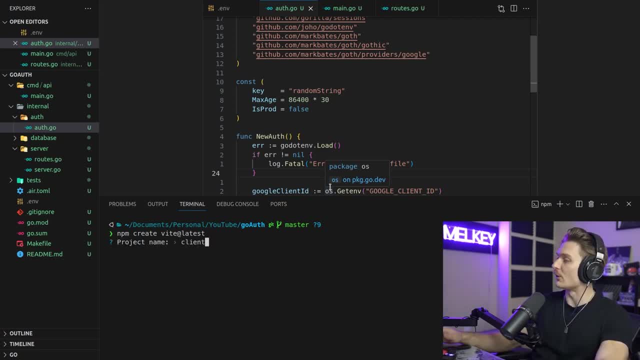 at latest command After you download it. I'm going to call our project, just our client, And here you can pick react, preact, lit, whatever I'm going to use react. We're going to use TypeScript, not server, not SWC, whatever that was, And I'm going to follow the instructions. 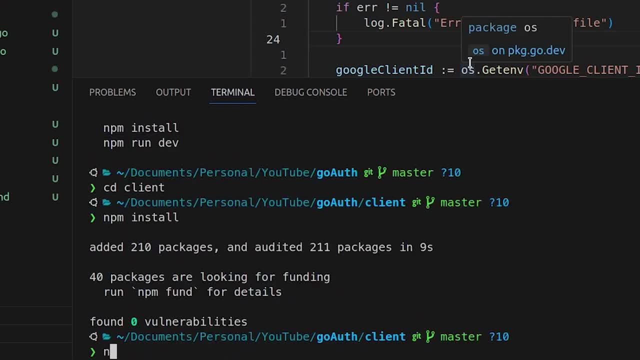 We're going to CD into our client. I'm going to run NPM install And next we're going to run NPM run dev And you can see here 51, 73,. that's the NPM run dev. And you can see here 51,, 73,. that's the. 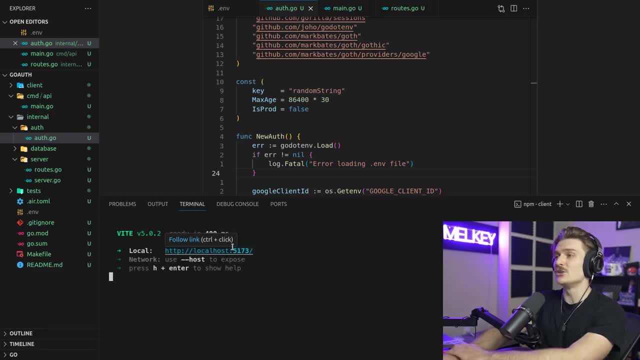 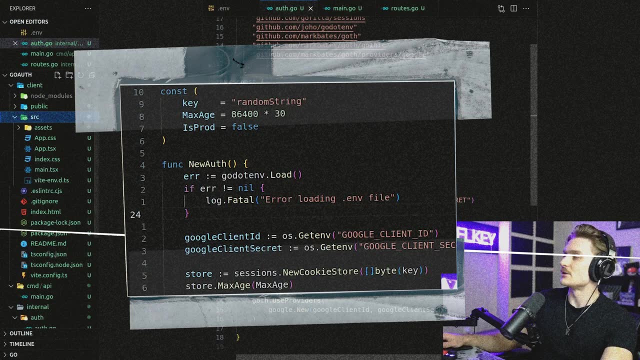 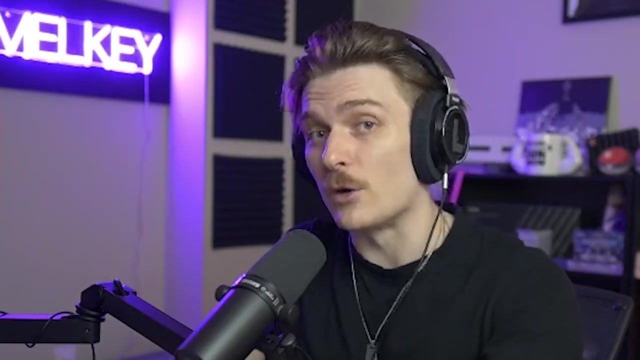 port, which we actually call for a redirect after a successful login. And if you just click this, there you go. We have a Vite app ready to go, All right. So now let's quickly just jump on over to react. our Vite app here, And we used to modify it. We have to just add a login function and log out. 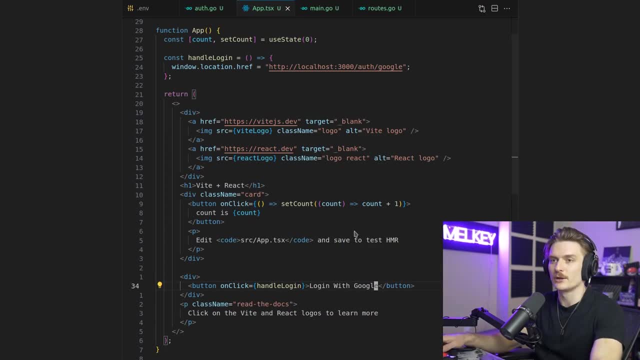 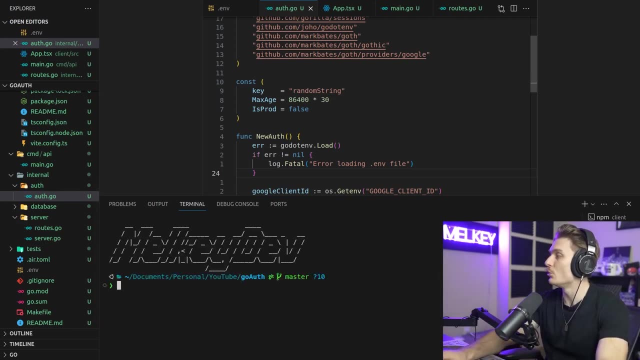 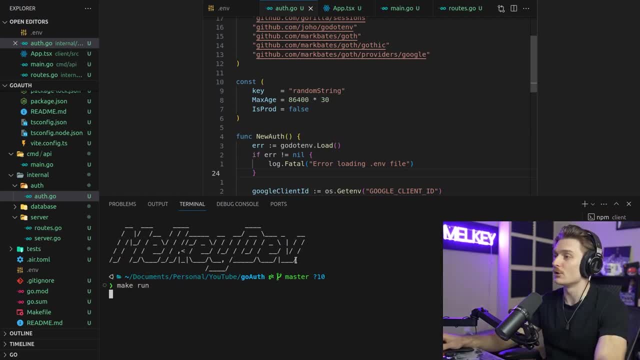 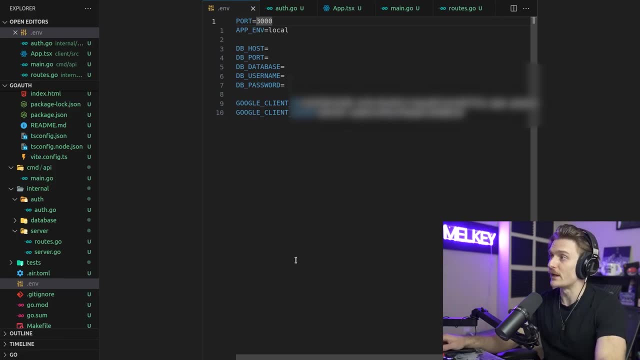 second terminal. all we have to do is click make run. This is going to launch our application, our report, which is defined in a inv file. I have set mine, for the purpose of this, to port 3000.. Again, Alex, you better edit these out. Okay, So now our application. 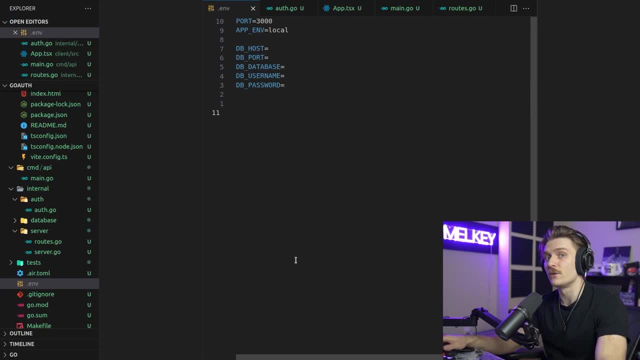 our backend is running on port 3000, while our front end is running on port 51, 73. And if I hop on over back to our local Vite app, it's now private incognito, because I don't want you guys. 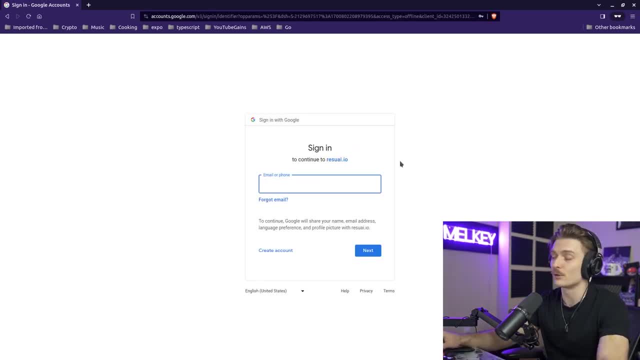 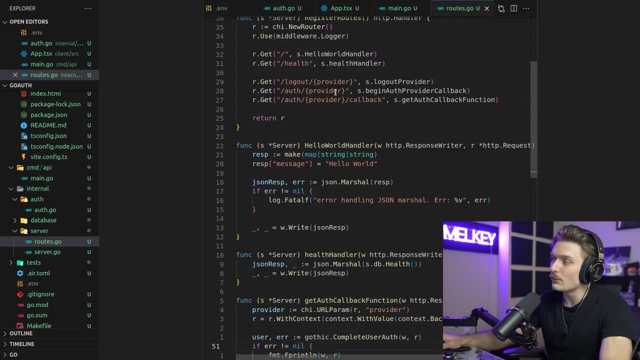 to see my emails. but if you log in with Google you can see. you can type in our email or phone number. it's going to prompt me to put in my password, click enter. so now we have logged in, but we can't really see it. how do we know? it worked well, if you remember back in our 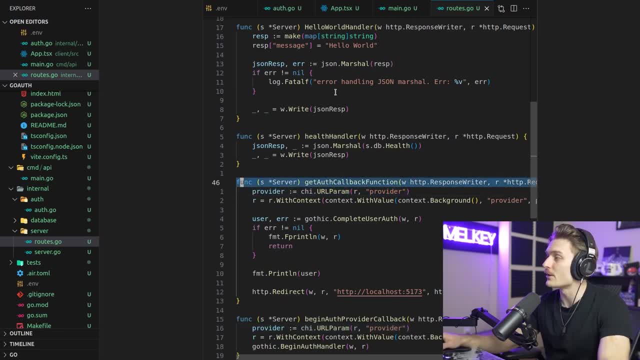 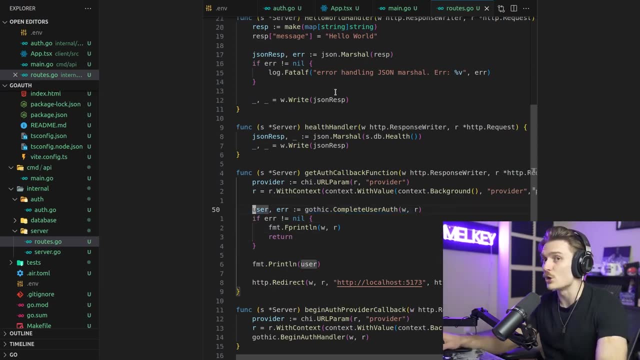 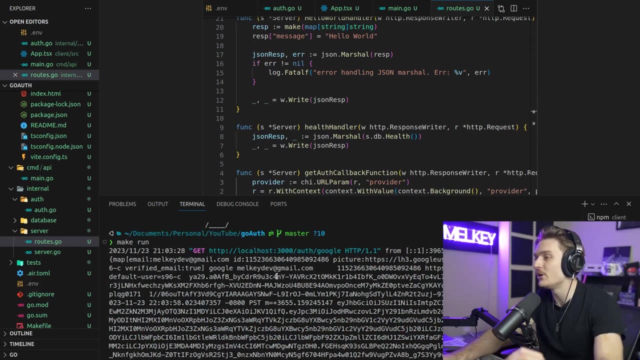 routesgo file here where we actually start the get auth callback function. we actually have a line here of printing the user after we complete the user auth from gothic and if we open up our terminal we'll look at what we have. we have the entire user struct from gothic and from google more. 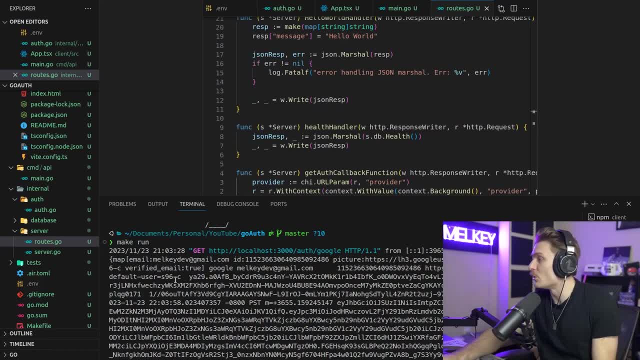 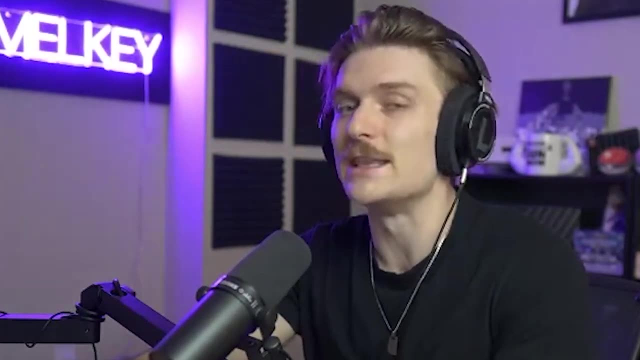 importantly. we have our email, we have the id, we have the picture. we have a bunch of information. we have the expiry of the token. all of that information is available to us to consume. through gothic, you can see the expiry of my refresh token. everything here is available to be used and this 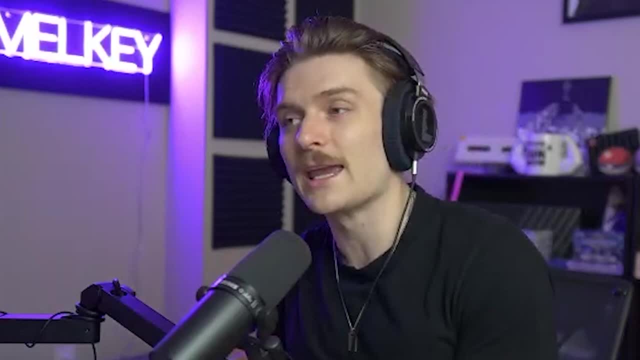 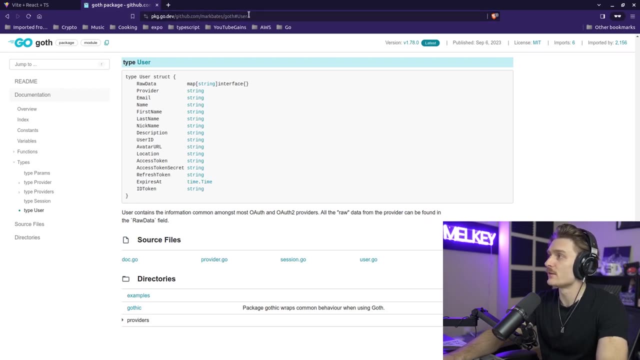 is how you actually use and structure oauth handling using gothic. now have this struct. now show you where you can find more information about this. you can see here over at pkggodev and the mark bates goth. you can see here that this user struct contains information common amongst most oauth and oauth2. 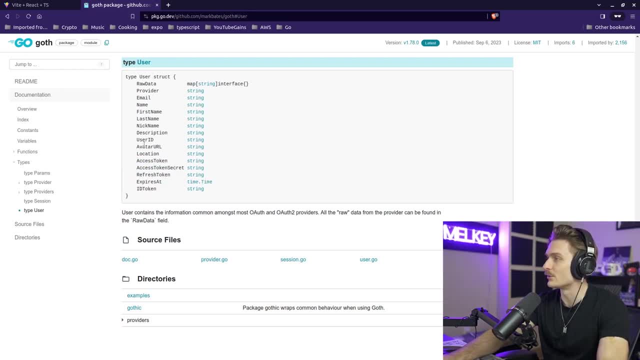 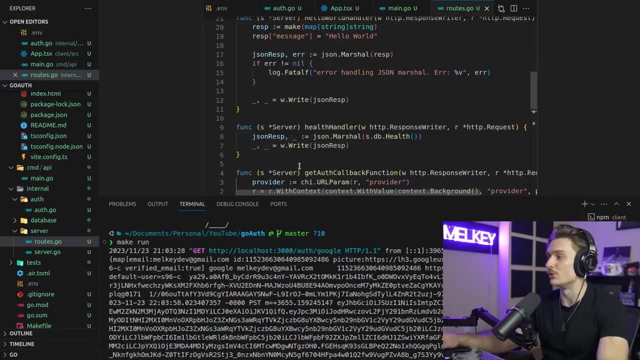 providers. you can see here the id token, refresh token, access token, location, avatar, user id. everything you need is going to be available in this user struct, which i printed in the terminal here below all right. so that was the entire breakdown, the entire tutorial, from start to finish.